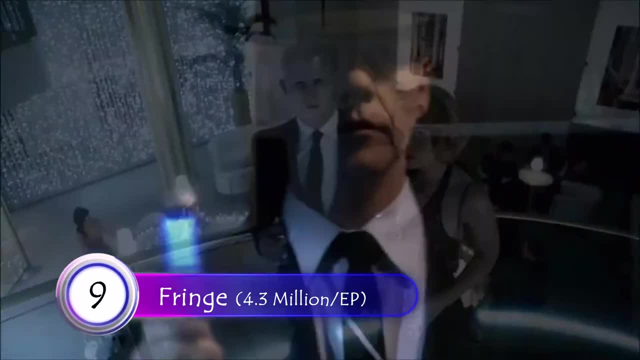 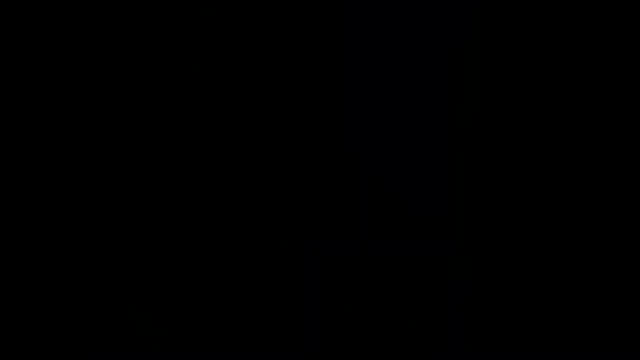 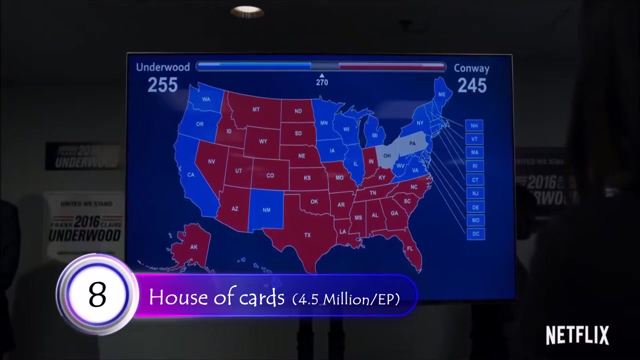 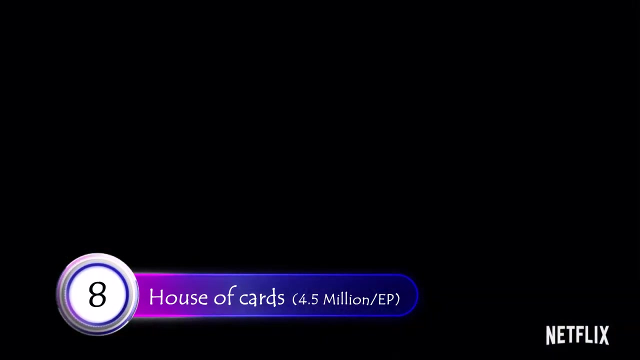 20 years. No wonder I'm so hungry. In the year 2609 AD, they finally ruined the planet. They even need help writing their wildest dreams, crafting their worst fears. Lucky for them, they have me, They have you. 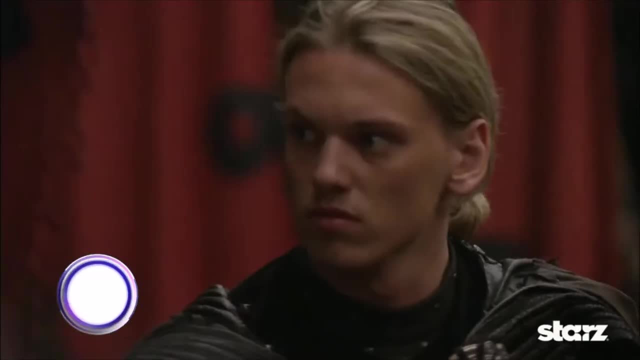 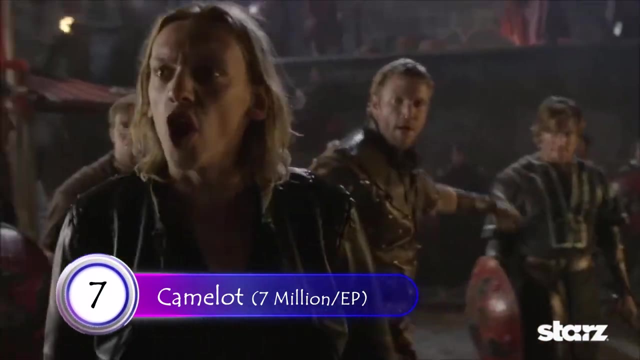 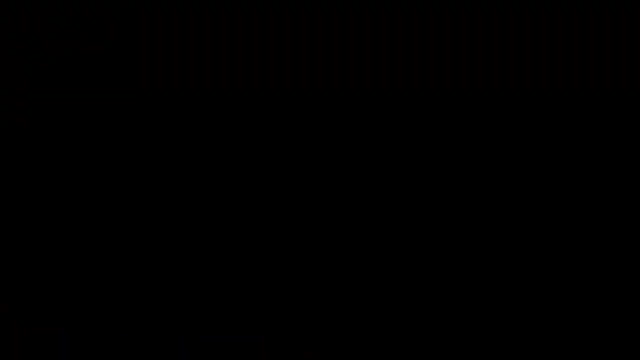 Everything you are is because of me. You will show me respect. Tomorrow could be the end of all of us. I will not be challenged. Answer your king, God, help me. So who is standing here? Who am I? Who am I? 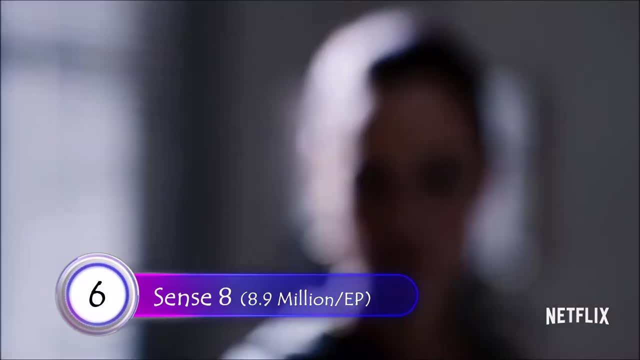 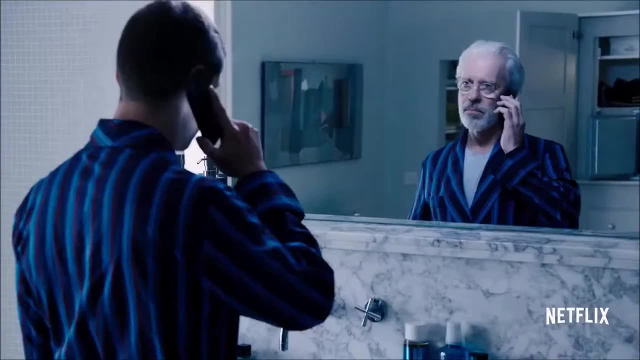 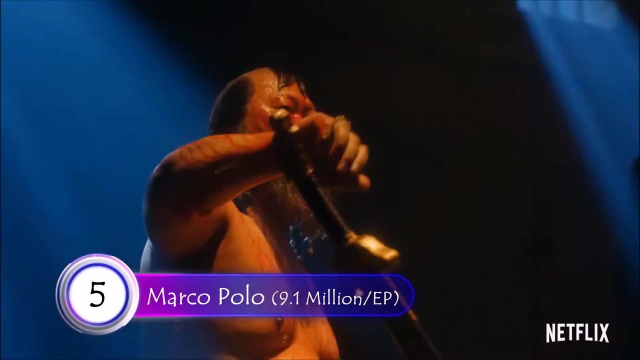 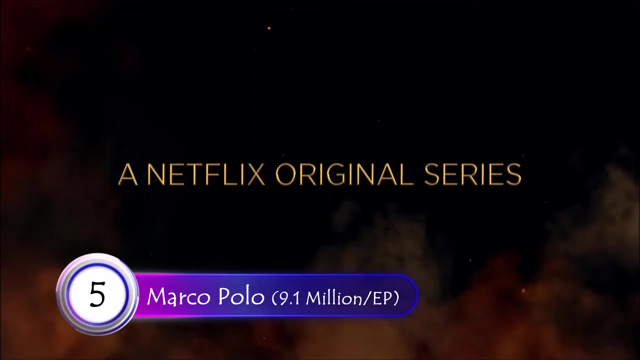 Do you mean where I'm from, What I fear? What do you mean What you see, What I've done with love? Who am I? punkt, Quote None and all discussed: I, I, I took the wall, I executed my brother. 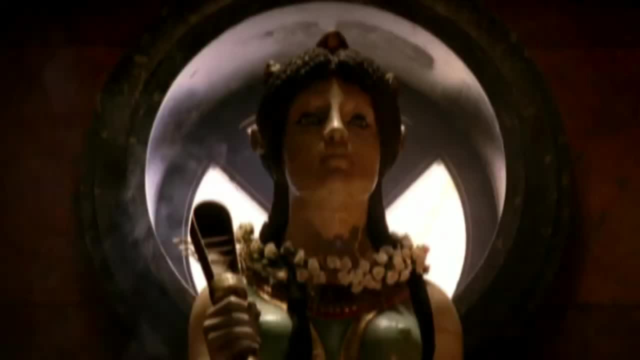 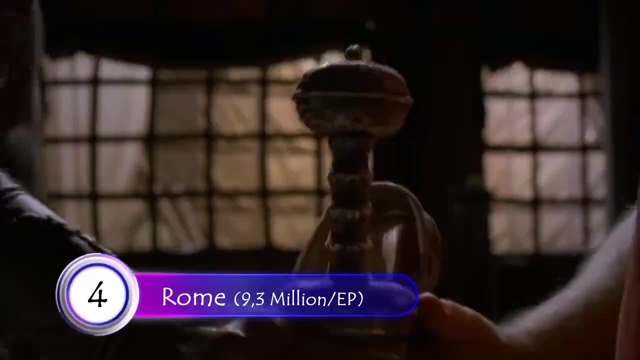 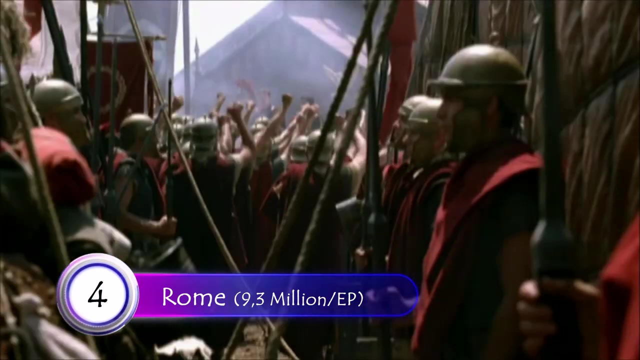 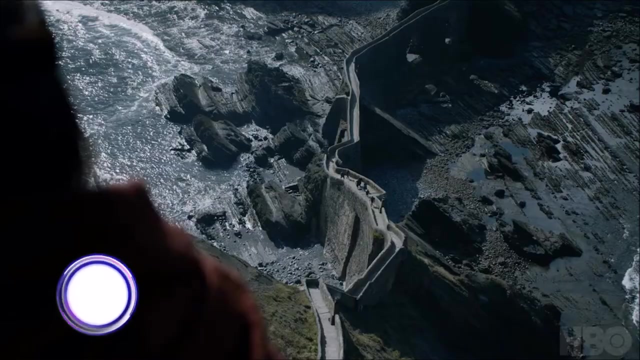 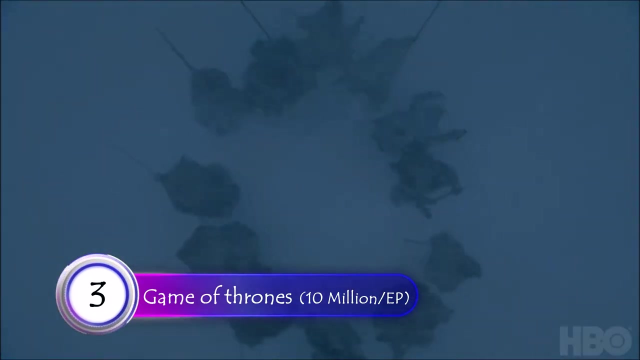 I do what must be done for our Empire By the spirits of my ancestors. I curse Caesar. The decisive battle begins. Caesar is now surrounded and severely outnumbered. Are you with me? Last best hope against the coming storm? If we don't put aside our enmities and band together, we will die. 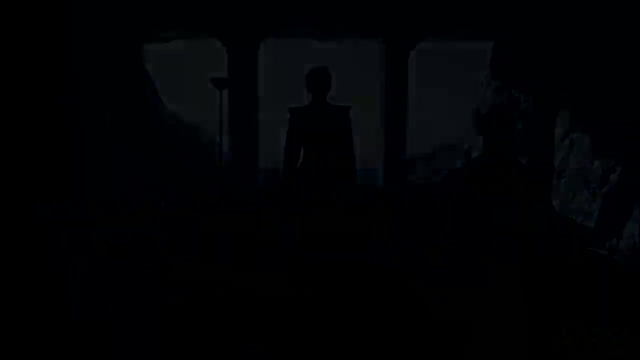 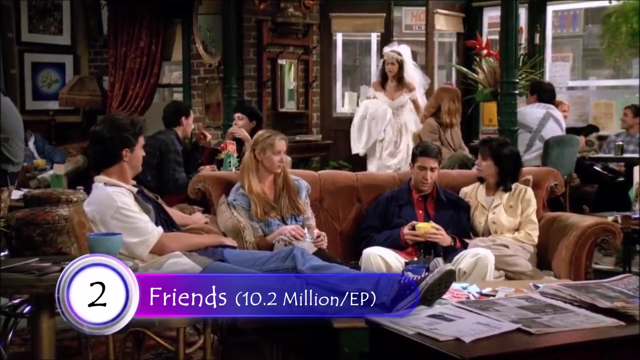 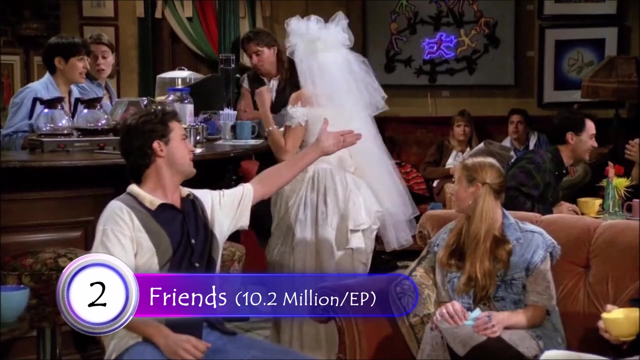 And then it doesn't matter whose skeleton sits on the Iron Throne. I don't want to be single, okay, I just want to be married again And I just want a million dollars. Great, Great, Oh God, Monica Hi. 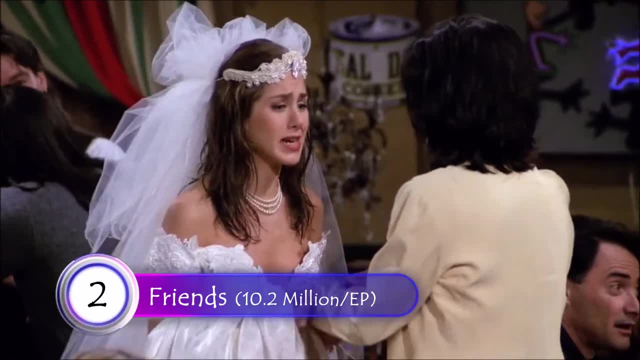 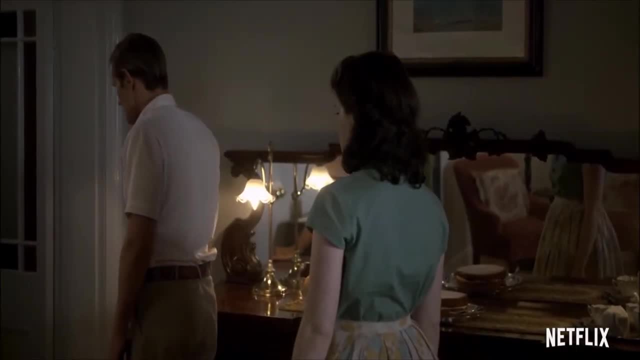 Thank God, I just went to your building and you weren't there, And then this guy with a big hammer said that you might be here. And you are, You are. Long live Queen Elizabeth. Don't you get sick of it all?